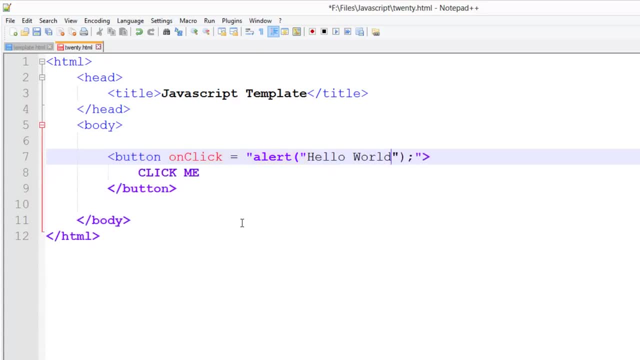 Now alert and we're going to go hello world. You're probably thinking we're on the 20th tutorial and we're still doing hello world. Yes, we are Right Now. you can see that we've got this syntax error here. This is going black, So it's basically showing that this is now no longer part. 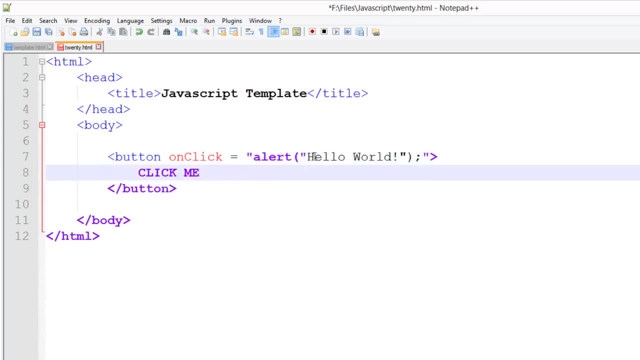 Of the JavaScript, Because the JavaScript you can see is supposed to be purple. Now, that's because the browser and Notepad++ will get confused about this And think that this is your code finished And it has no idea what this is. And then suddenly you start another set of double quotes. 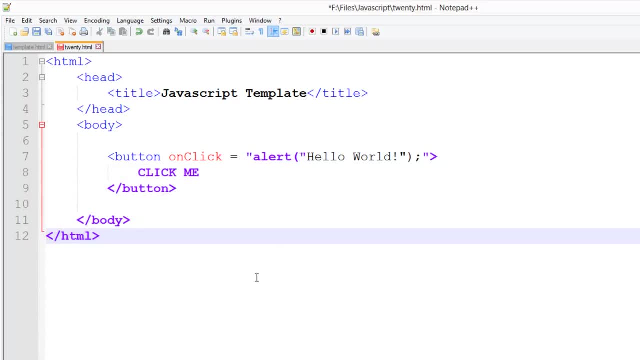 And you never finish it. So JavaScript allows us to use two types of quotes. We can use these ones, Which is the double quotes, And we can also use these ones, which are the single quotes, And HTML doesn't understand these single quotes, So we can use those to kind of bypass this issue. 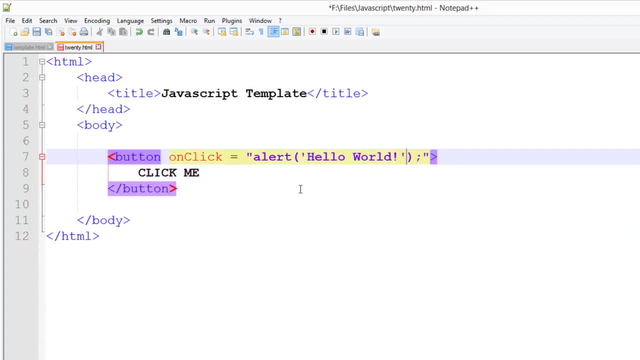 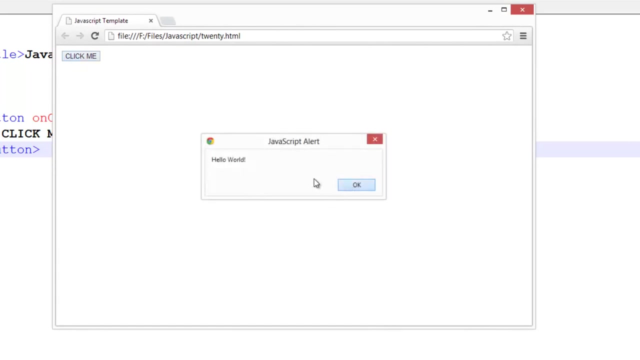 So we can put a single quote here And a single quote here And JavaScript will recognize that, But HTML won't. So you can see all of our formatting. our syntax is much better now. So now, if I save this and run it And we press click me And you see the button is the pop up box comes up. 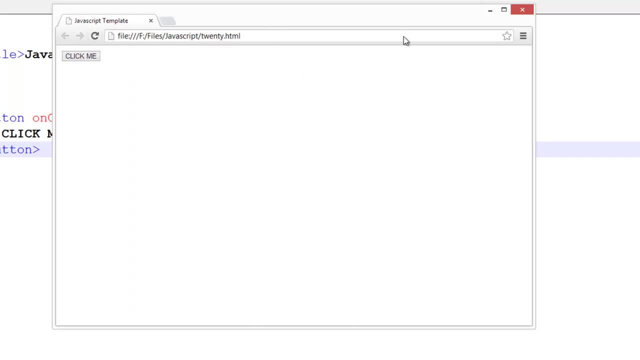 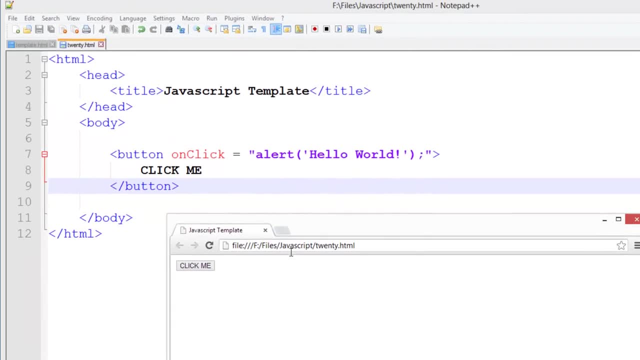 Before this would have happened on the on load event And that's why, when you refresh, you would have got the pop up box straight away, Which is not what we want. So there's a couple of other ones we can use. We can use on mouse over. 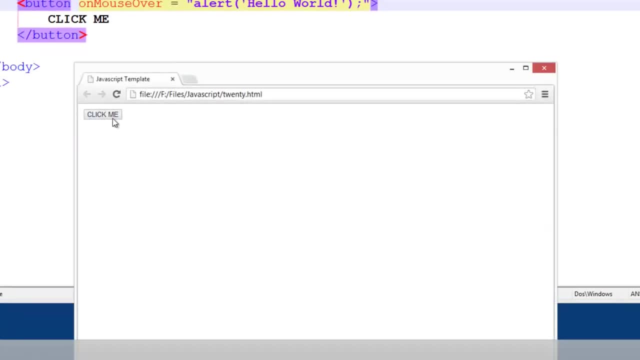 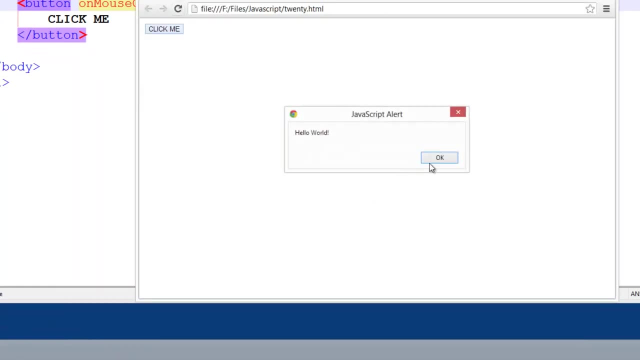 We can save that And launch it in Chrome. You can click me. Oh, I didn't even need to click that. I made a mistake. If I refresh that and I hover over it, I didn't click. You can hear me clicking. 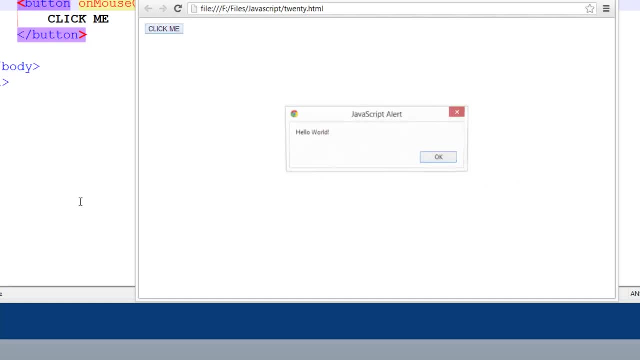 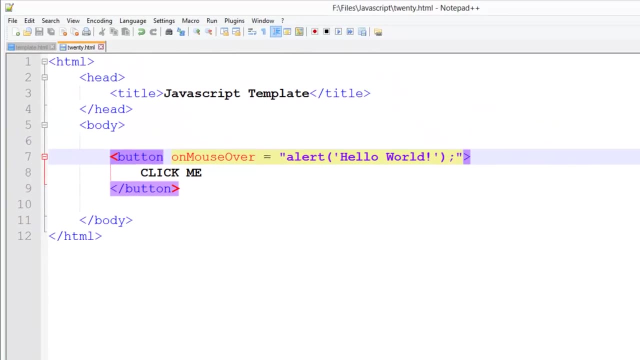 And you see, it's just going straight over. I can go straight over and it does it. I'm not going to show you how to use all the different events. I'll put a list of them. You can try them all out. You're basically just replacing this with the event name. 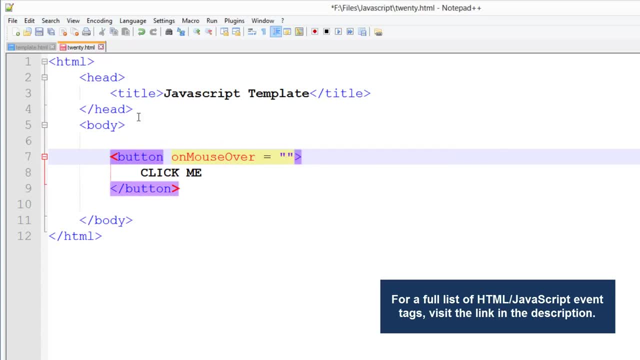 So now I'm going to show you something else: How you can use this. What we can do up here is we can create a script tag And script type equals text Slash- I'm not supposed to say CSS, but Javascript- And then close off the script. 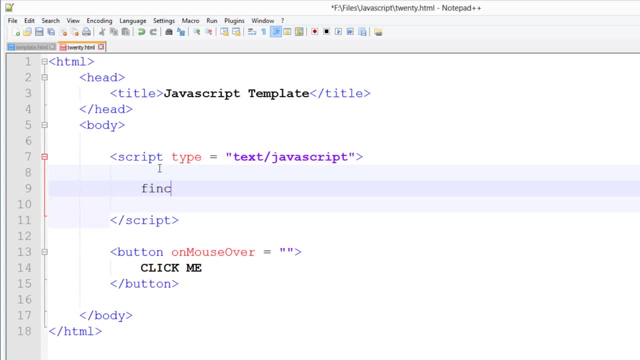 And then what we're going to do in here is we're going to create a function, So we're going to go function, Not function Function, And we'll call it button press, Put your brackets and your curly brackets, And here we're just going to do alert. 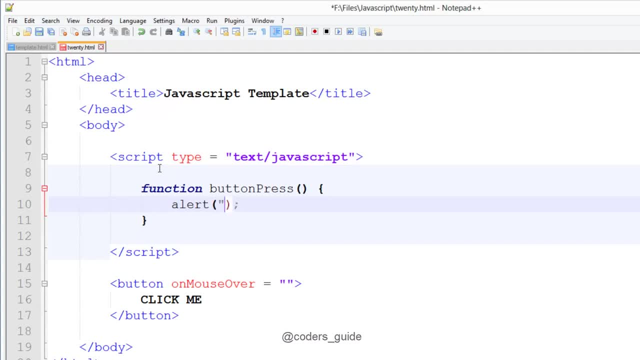 And As the text will just go higher, Like that, And we'll duplicate this as well and go higher, So we're going to be doing two pop up boxes here, Then here. since this is just Javascript, we can simply go button press. 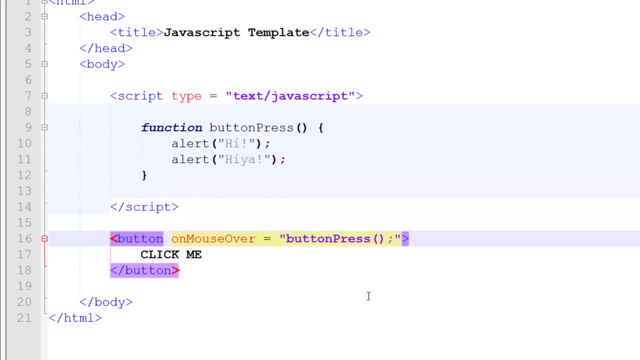 Put your brackets and your semicolon. So this is basically just kind of when this is mouse over, When you hover over it, We're going to go button press And we're going to launch this Javascript code which is telling us to launch this function. 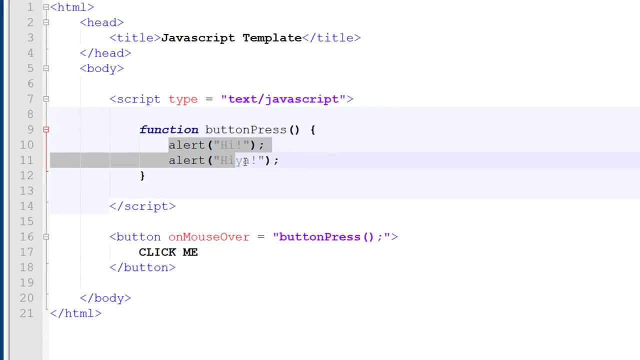 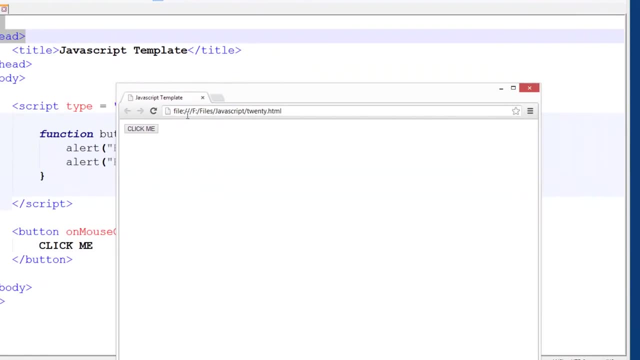 So we're going to go over here. Here's the function And we're going to do this code. So I'll just zoomed up. We're going to run in Chrome And we hover over it and it comes up saying hi. 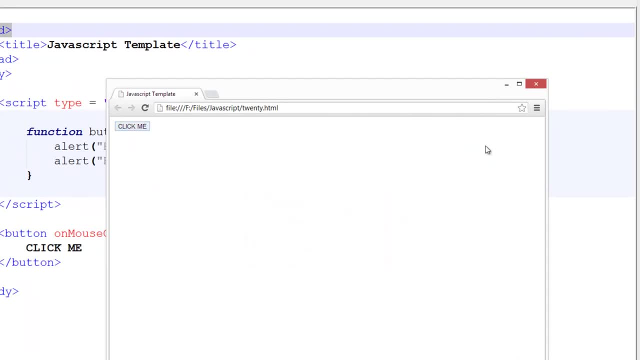 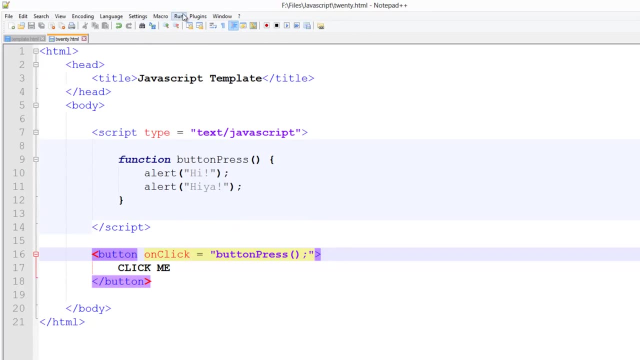 Higher, So you hover over it and it comes up with those two boxes. So we can also do here on click obviously, Just like that, And you know, when we click on it we get the two boxes. One more thing that we can do is we can also put more than one thing in here. 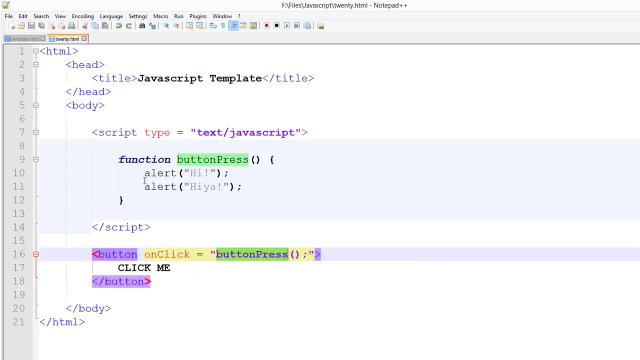 So we can. in Javascript we might put all these separate lines, So you put this here, Then we put the semicolon, Then we go onto another line, Although this will still work if we have it all in one line. So we can use that to our advantage. 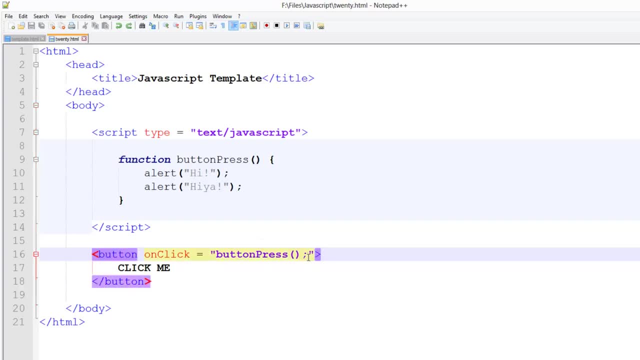 We can go button press, Put the semicolon And then we'll also go alert. Um, Hello, Just like that, And don't forget your semicolon. And don't forget to use single quotes as well. So now, if we save that,